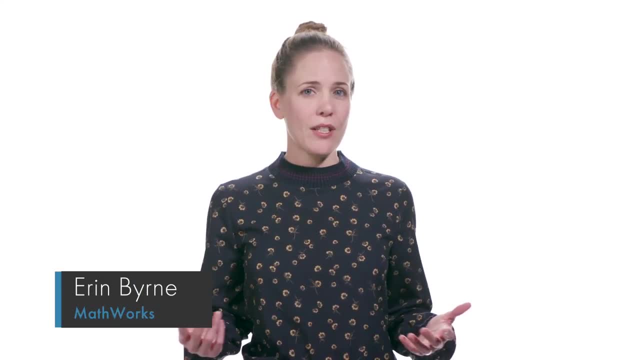 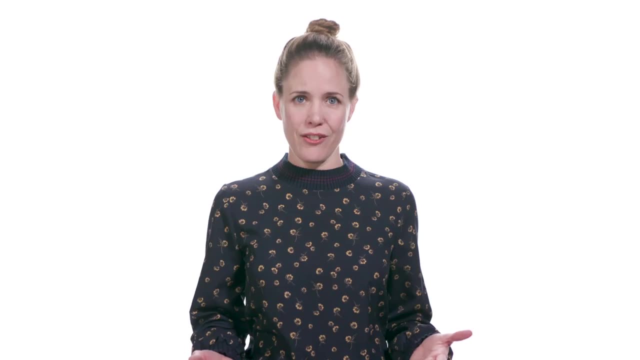 We live in a world of sensors. They're in robots, in factories, in our cars, on our wrists, even in our refrigerators, making sure our food stays fresh. These sensors generate signals. In this video, we'll use Simulink to process a signal from a sensor. We'll perform spectral. 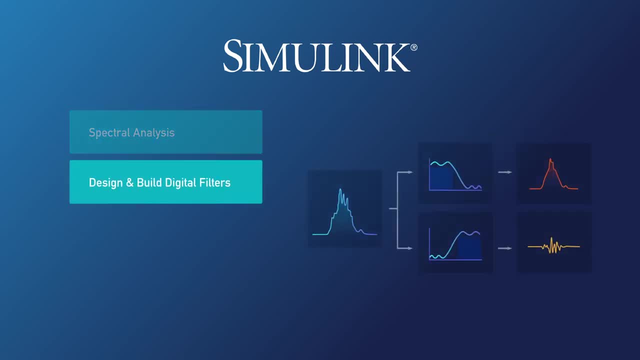 analysis to explore the signal. Based on that, we'll design and build digital filters as part of a signal processing algorithm. We'll assess the performance of our algorithm and, once it's ready, convert our model into C code that can be embedded into real-time hardware. 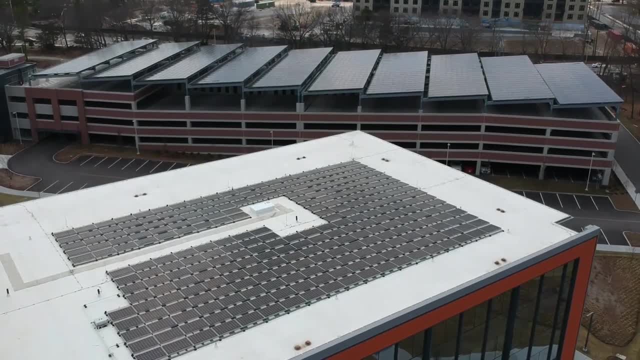 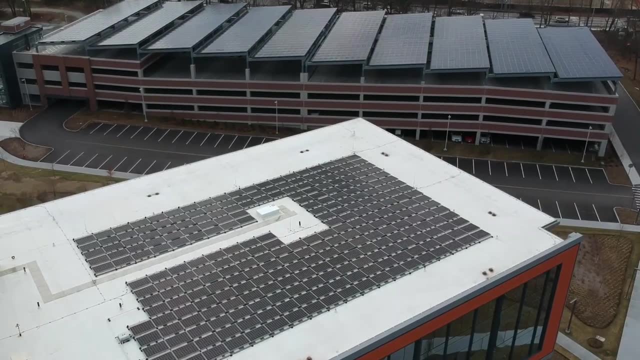 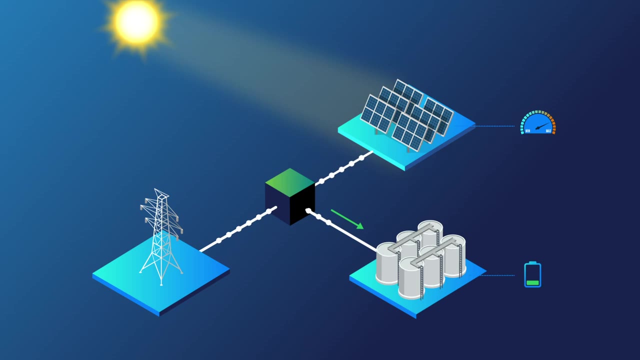 So let's get started. At the MathWorks headquarters in Natick, Massachusetts, there are solar panels that generate electrical power. We'll use measurements of the power produced by the array every 15 minutes. This is our signal. Of course, the power depends on the amount of sunshine. 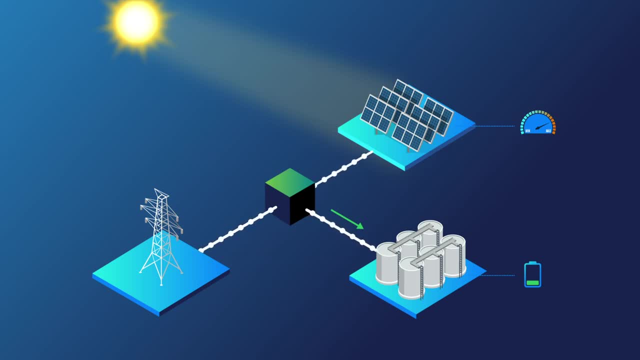 which depends on the time of day and the weather. Predicting and managing the variable production and demand is an important part of renewable energy generation. To smooth out the generated power, on sunny days we can store some of the power in a battery. Then on cloudy days, we use it to supplement the lower power. 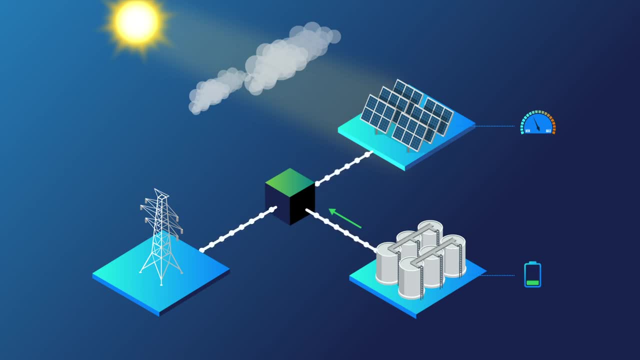 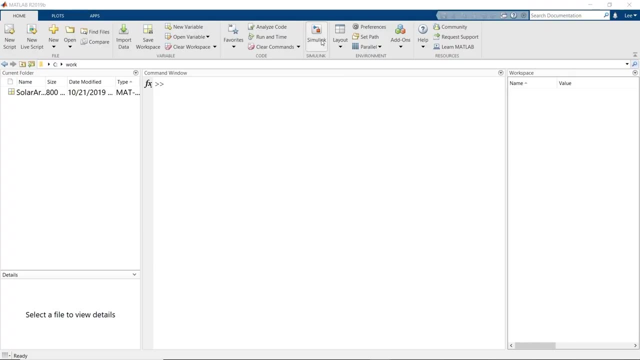 generation. Let's design a system that can predict if it's going to be sunny or cloudy using signal processing techniques in Simulink. You start Simulink by clicking the Simulink button on the MATLAB tool strip. This opens the start page where you can create new models. find examples. 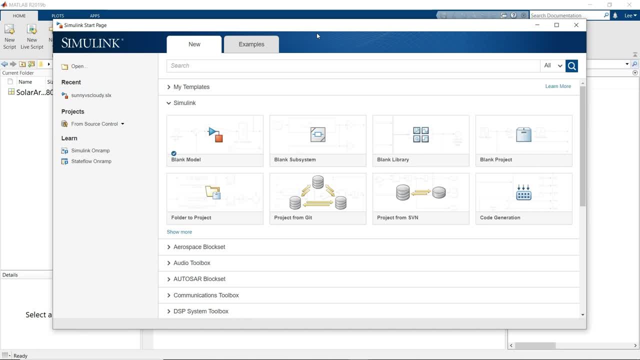 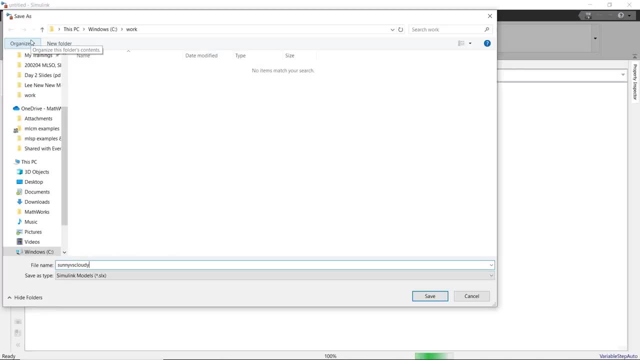 and even find basic training. We're starting our model from scratch, so we'll choose Blank Model and save it as Sunny vs Cloudy Simulink models are built up from blocks and signal lines. Open the library browser to see all the blocks available. 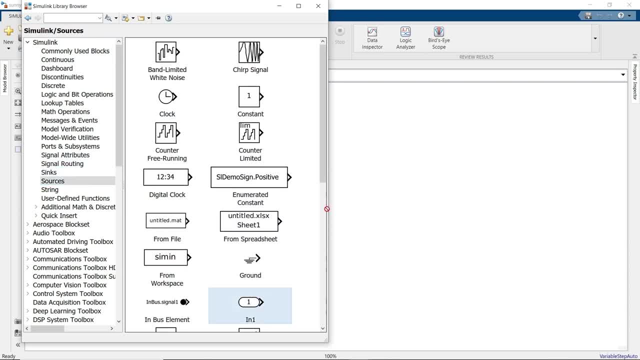 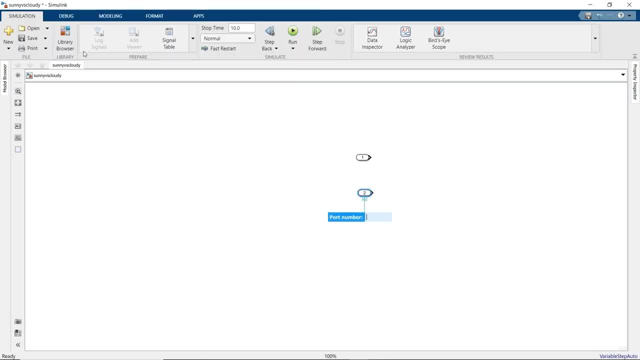 We'll start by visualizing two power signals, one from a sunny day and one from a cloudy day. To view our signals, let's drag two input ports- or IN ports for short- into our model, Then add a scope block. 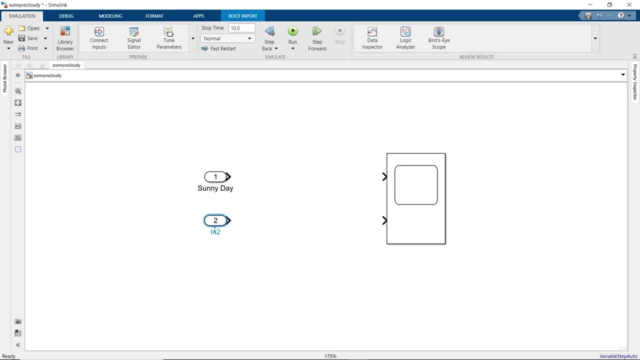 Let's label the two IN port blocks- Sunny Day and Cloudy Day- and the scope block Time, Domain. We can connect the blocks together with signal lines by clicking and dragging To label the signal line, double-click and type the name. Now we need the data. In MATLAB we have two vectors: Sunny Day and Cloudy Day. 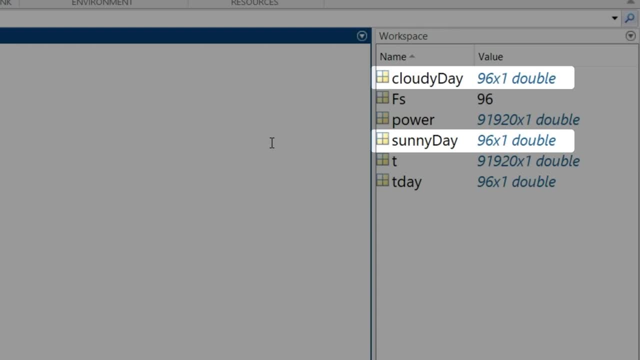 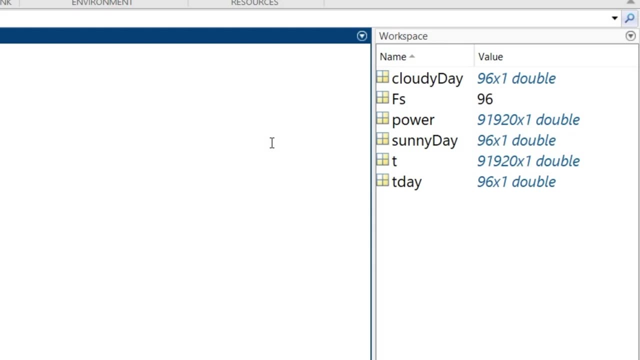 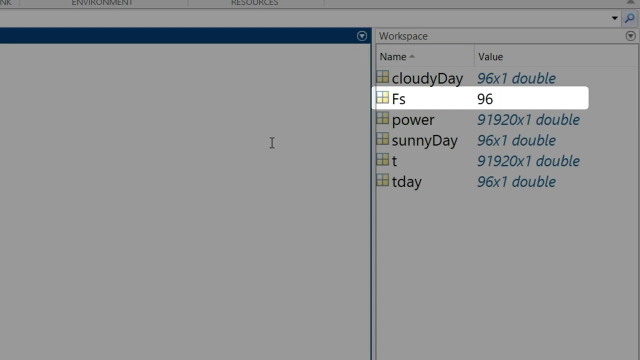 representing the power measurements for two particular days in June. The corresponding timestamps are in T-Day. We also have the sample frequency in Samples Per Day in the variable FS. Sampling every 15 minutes means that we get 96 samples per day. 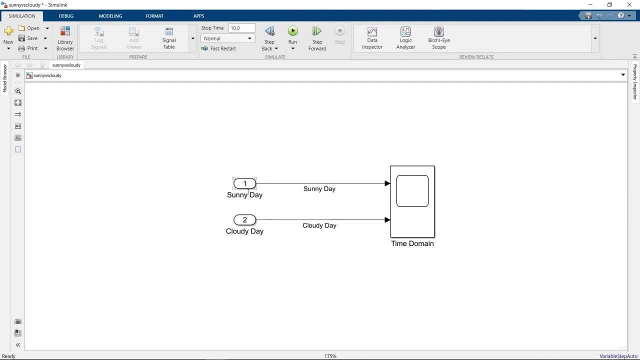 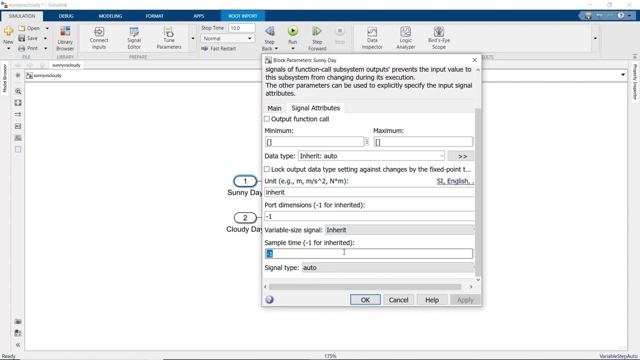 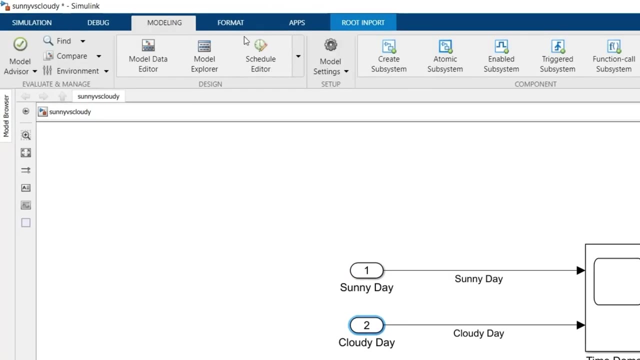 We have to set the sample time of the two IN ports. so double-click on each IN port to adjust its block parameters. Under the signal attributes tab, set the sample time to the reciprocal of the sampling frequency To bring the data into Simulink. we can go to the Model Settings tab. 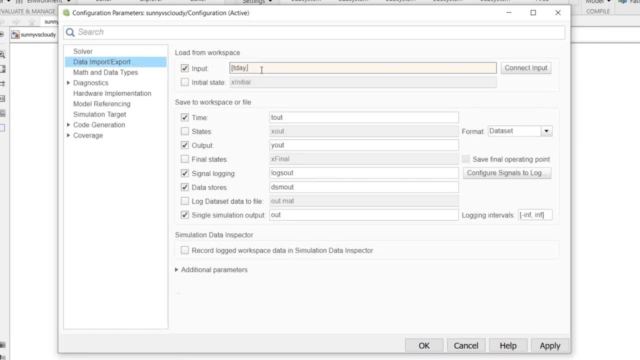 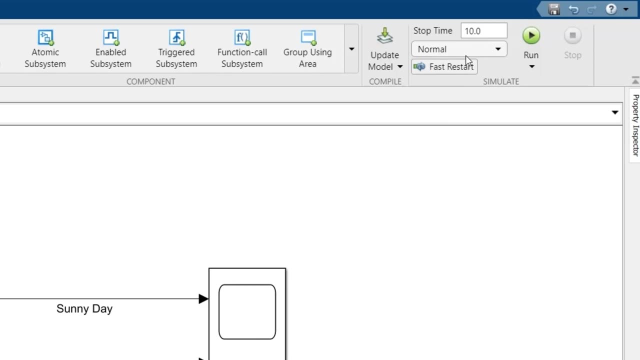 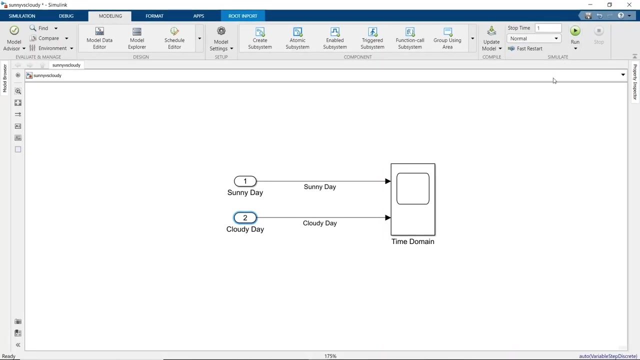 Settings window, then the Data Import- Export pane and add the time and two power signals as inputs. We should also set the total simulation time to one day. We can now run our model by clicking on the Run button in the tool strip. Let's double-click on the scope block to see the signals and let's connect our data. 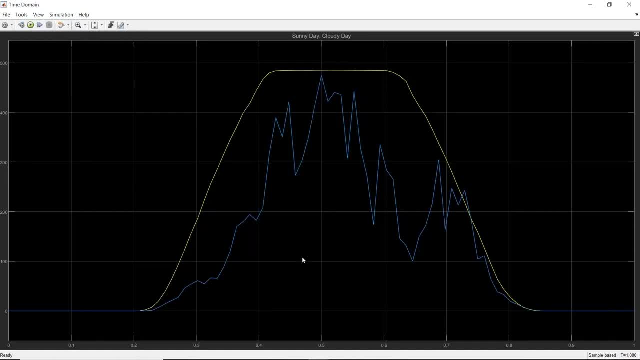 points using lines. The smooth yellow line is the sunny day. The blue line shows that the cloudy day produces less power, as you'd expect, and also has many short-term variations as the clouds pass over the solar array. So how can we use these features to decide if we have a sunny day or a cloudy day? 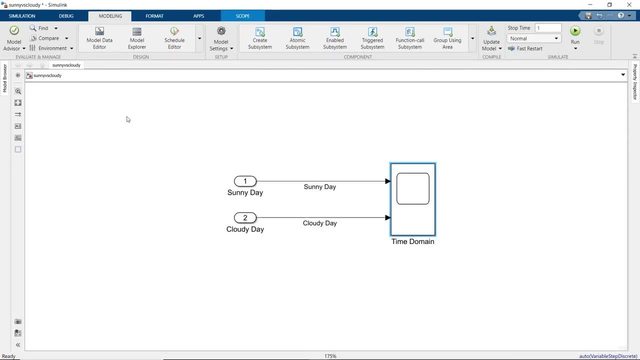 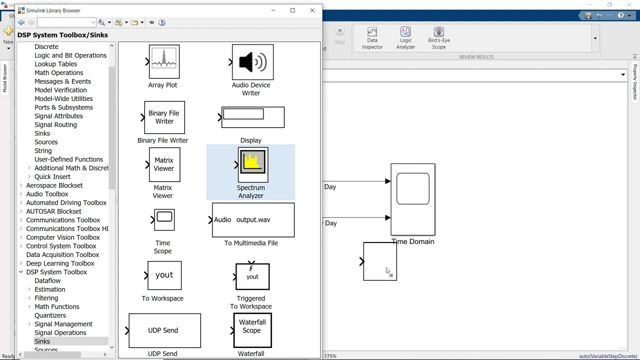 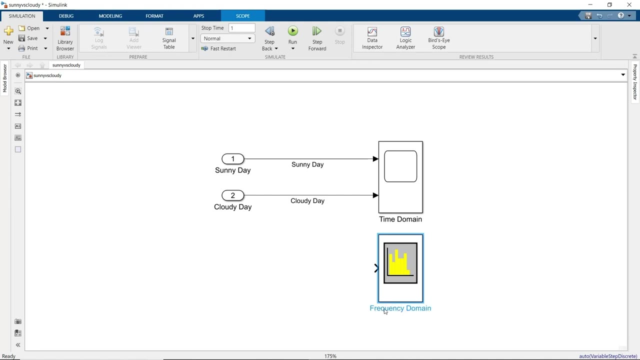 Well, let's also look at these signals in the frequency domain. We'll use spectral analysis, which helps us measure the frequency content of each of the signals. We first add a spectrum analyzer block from the DSP system toolbox And then connect the two signals to it. 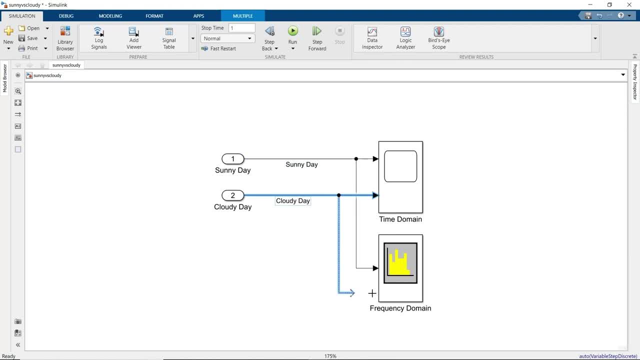 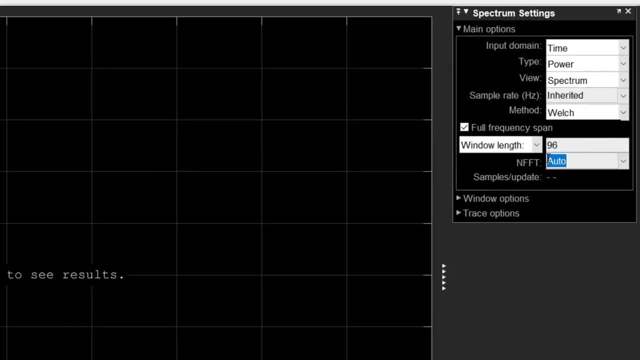 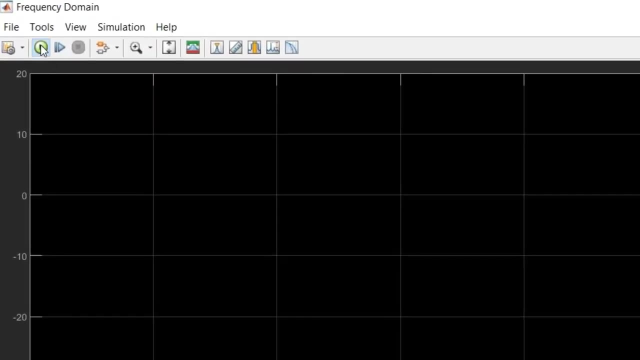 To branch a signal line. you can right-click as you drag the signal line to a block. We have short signals, so we'll need to change a few settings in the spectrum analyzer block so we can see them properly. This time we can run our model from within the spectrum analyzer by pressing the green. 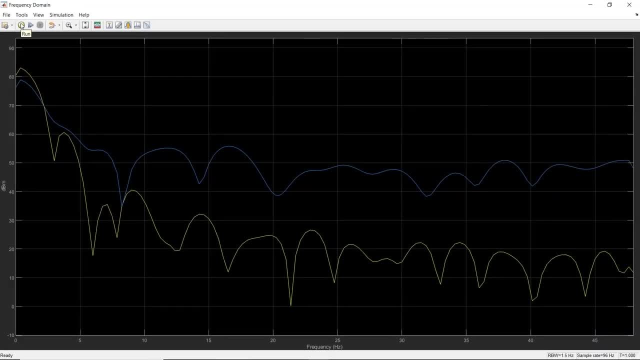 button at the top. Let's turn on the legend to see which day is which. So what are we looking for? What are we looking at? The x-axis is the frequency value. The y-axis shows us how much power is in our signal at a given frequency. 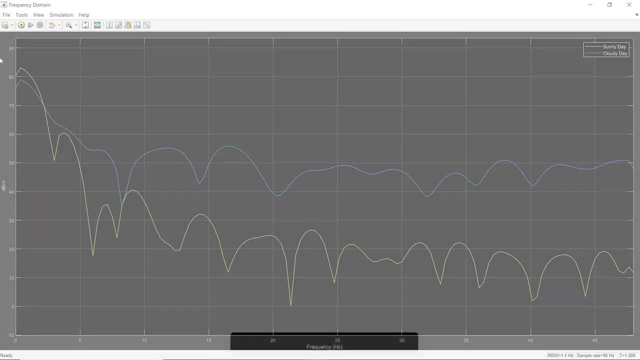 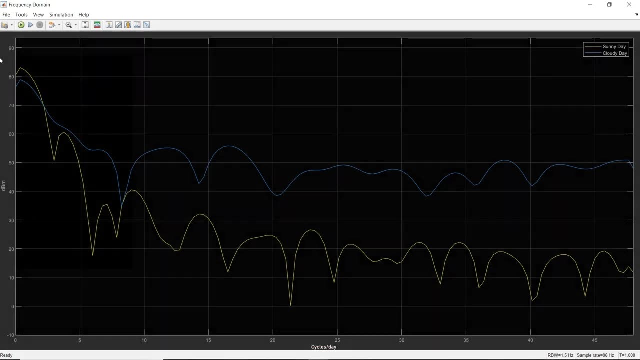 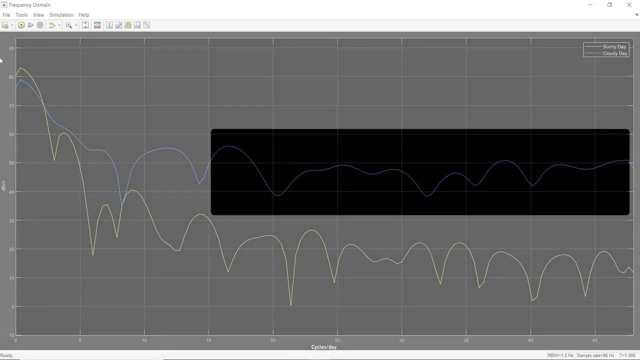 Although the default time unit is seconds, we're actually measuring time in days, so the x-axis is cycles per day, not cycles per second or hertz. We see that the low frequency content is about the same for both days, But the cloudy one has way more high frequency content. 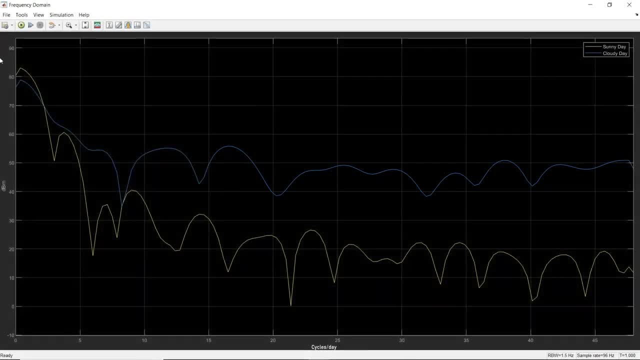 Remember those short-time variations? Well, that's how they look in the frequency domain. So maybe we can tell sunny from cloudy by comparing the power in the higher frequencies to some threshold. However, the panels produce more power in the summer and less in the winter, which means 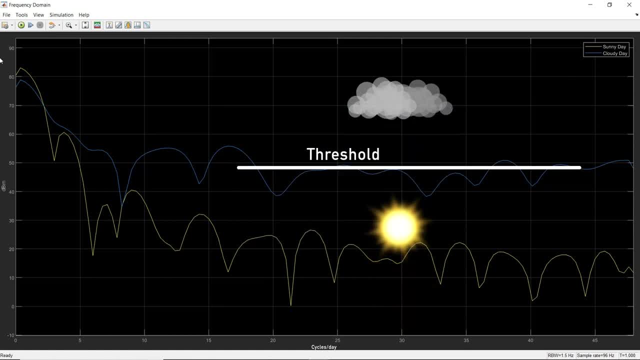 the threshold would have to change throughout the year. Well, we'd like to have a constant threshold for all seasons of the year. If we normalize the high frequency power by the power in the lower frequencies, we can use a fixed threshold. So let's try computing the ratio of the total power in the top 75% of frequencies to the 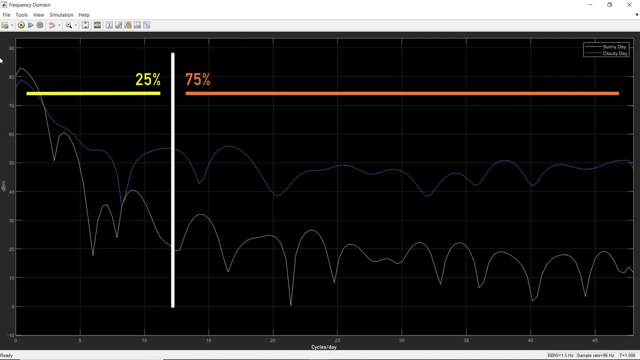 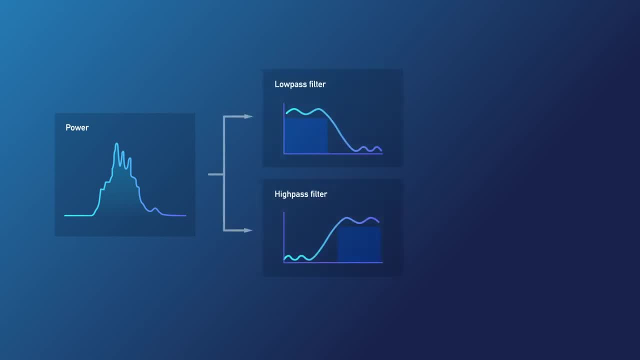 total power in the bottom 25% of frequencies. So how do we separate the low and high frequencies? By building digital filters. We need a low-pass filter for the low frequency content and a high-pass filter for the high frequency content. To build these two filters, we first strip our model back. 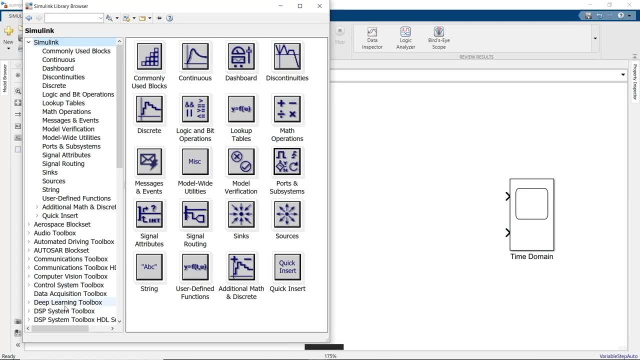 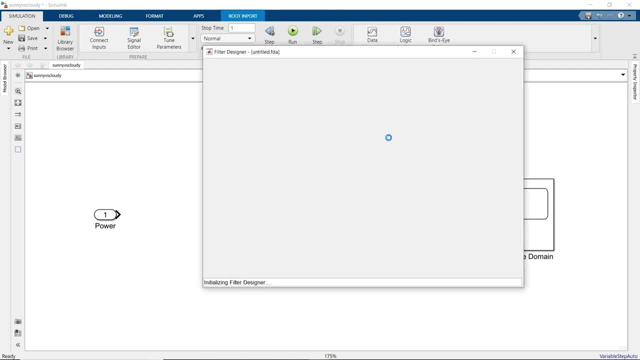 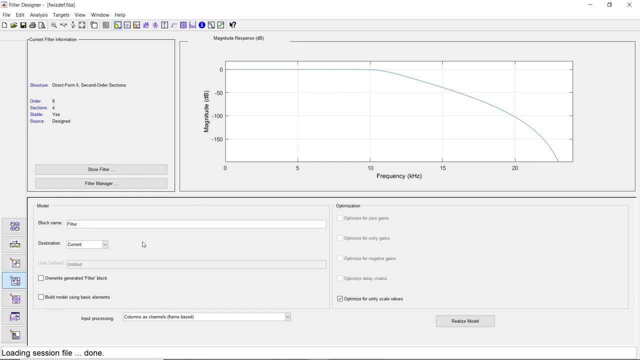 To a single import and scope block And drag in a filter realization wizard block from the DSP system toolbox. Double-click the block to open the filter designer app. If you've designed filters in MATLAB, you may have used this app before. Let's click on the design filter icon to start designing the low-pass filter. 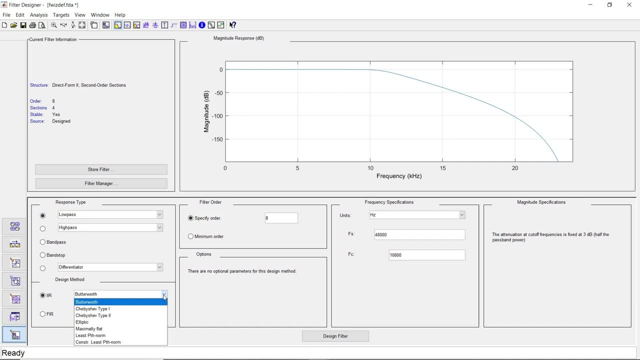 Because we only get samples every 15 minutes. we need a filter that can work with just a few samples. We'll use a Chebyshev Type 1 IIR filter and we'll set the filter order to 4.. We then have to specify a cutoff frequency. 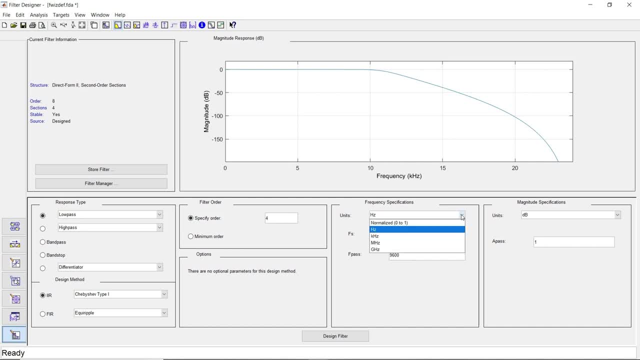 Remember we wanted to let through the lower 25% of the frequencies. So we'll select Normalized Frequency and set Wpass to 0.25.. And we'll keep the passband ripple to less than 0.05 dB. Finally, push the Design Filter button at the bottom. We see that the new response is 0.05 dB And we'll keep the passband ripple to less than 0.05 dB. Finally, push the Design Filter button at the bottom. We see that the new response is 0.05 dB. And we'll keep the passband ripple to less than 0.05 dB. And we'll keep the passband ripple to less than 0.05 dB And we'll keep the passband ripple to less than 0.05 dB. 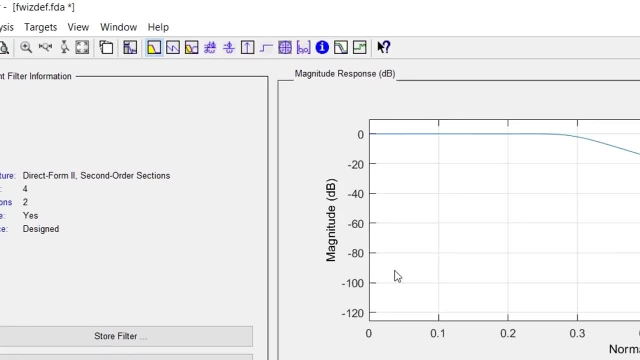 We can examine the delay introduced by our filter by clicking the Group Delay Response button. We can examine the delay introduced by our filter by clicking the Group Delay Response button For frequencies less than 0.25,. the delay is about 3 samples. 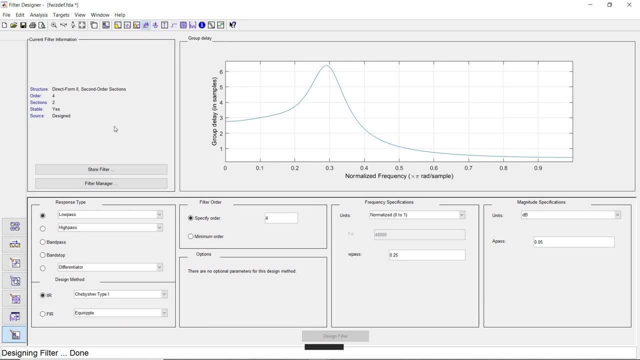 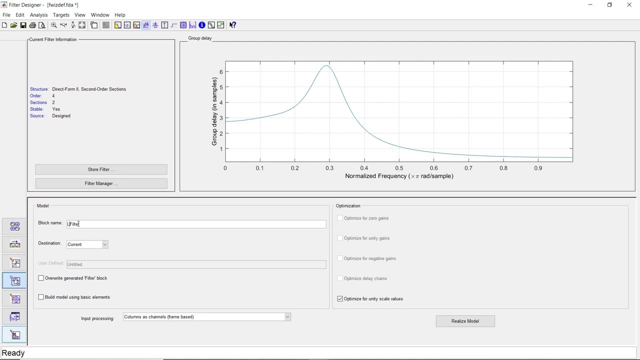 Let's remember that for later. Now that we're done designing the filter, let's add it to our Simulink model by clicking the Realize Model icon. We'll call the block Low Pass Filter and select the option Build Model Using Basic Elements. 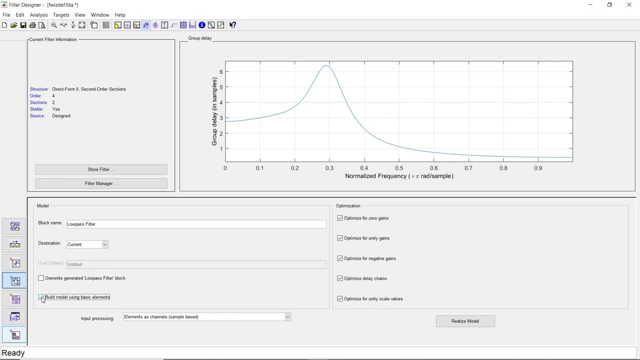 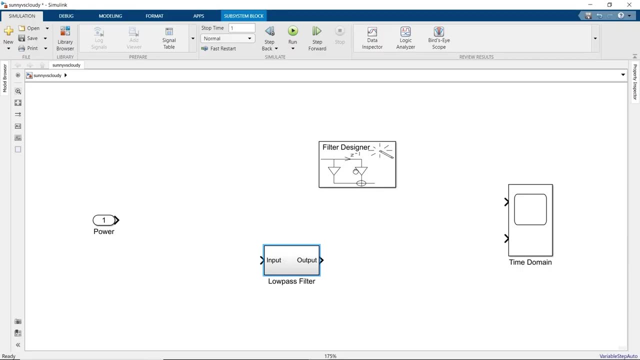 That way we can see the basic Simulink blocks used to make the filter. that way we can see the basic Simulink blocks used to make the filter, Like Delay, Multiply and Add blocks. When we click the Realize Model button, a new subsystem is created in our model. 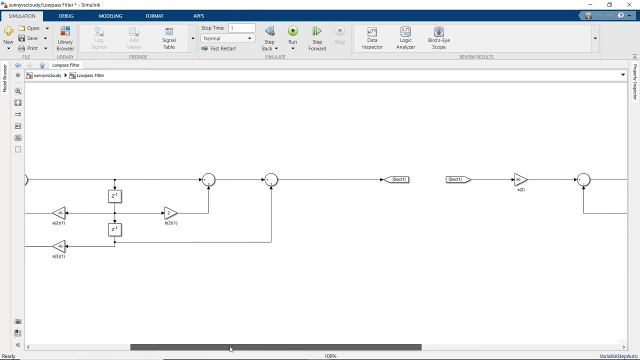 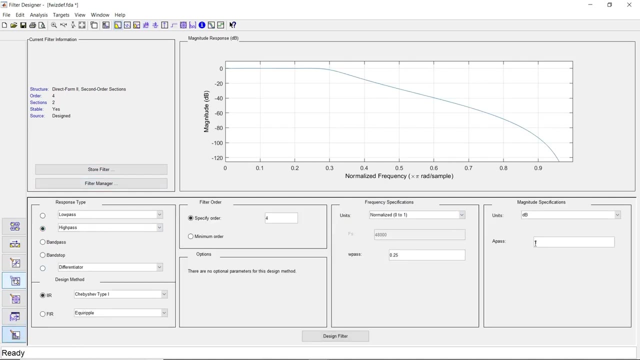 Let's double-click this to look inside. Sure enough, the filter is just Unit Delays Gains and Add blocks which modern DSP chips and FPGAs are optimized to implement. Now for the High Frequency content. Well, we can repeat the same process to design and realize the High Pass Filter. 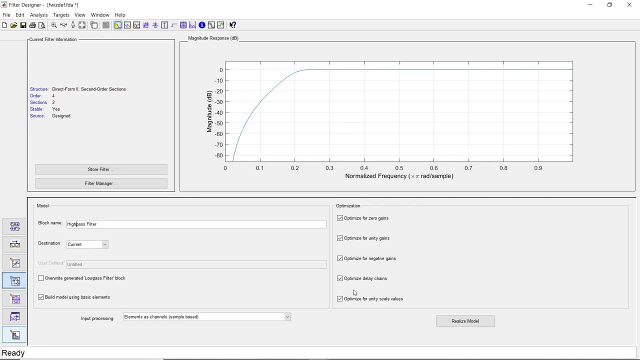 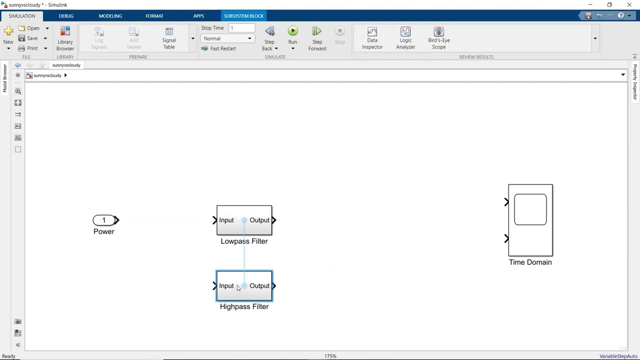 In this case, the High Pass Filter delays the input signal by one sample. Okay, let's test our new filters on the power signal. We had three parallel paths: one for the original power signal, one for the Low Pass Filtered version. 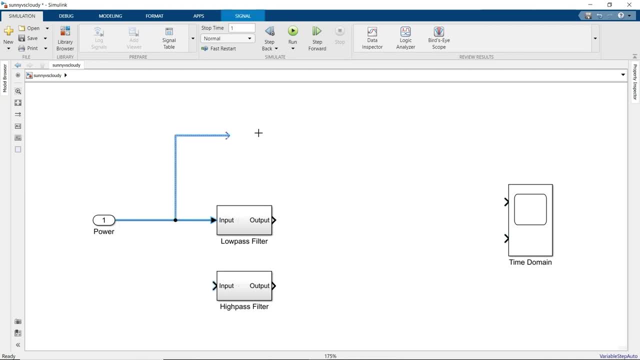 and one for the High Pass Filtered version. We want to compare them, But remember that the Low Pass Filter introduces a delay of three samples and the High Pass Filter introduces a delay of one, So we need to add some delay blocks to make sure the three signals are aligned. 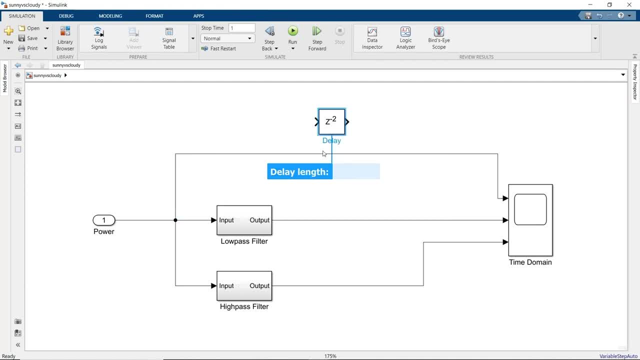 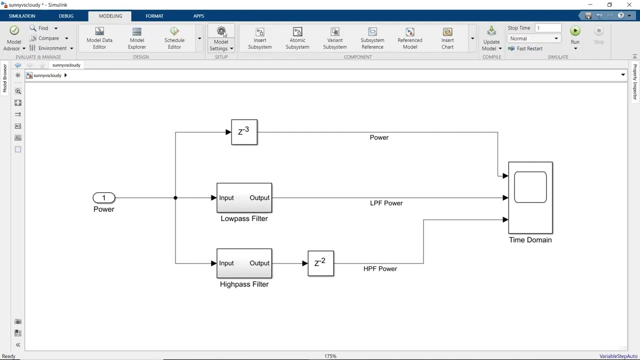 double-click on the model and type Delay to quickly add a delay block to the original signal of three samples and another delay block to the High Pass signal of two samples And we'll modify the model to work with a much longer- two and a half year- data set that we have. 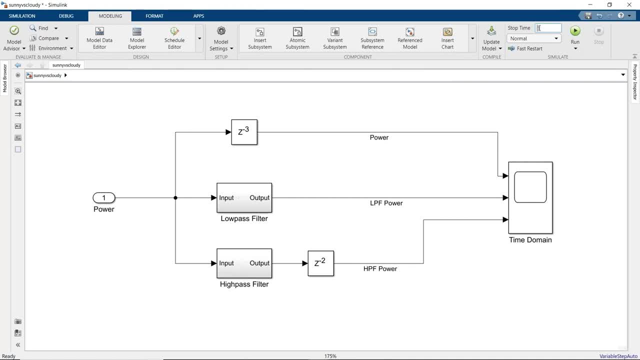 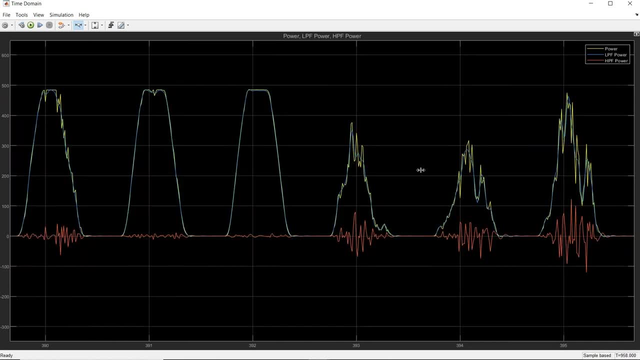 which is stored in the variable Power, with timestamps in T On the scope. let's zoom in on six days. The yellow line is the time stamp and the blue line is the time stamp. The yellow line is the time stamp and the blue line is the time stamp. 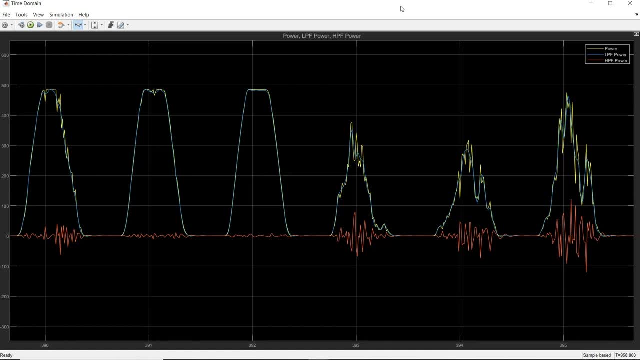 The yellow line is the time stamp and the blue line is the time stamp. The yellow line is the original power signal, The blue line is the low pass signal, which represents the general smooth trend, And the red line is the high pass signal which captures the variations due to cloud cover. 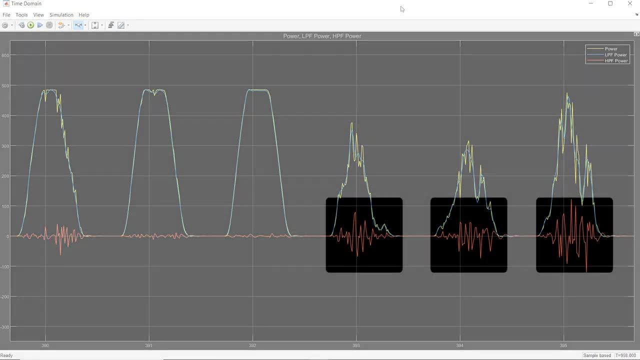 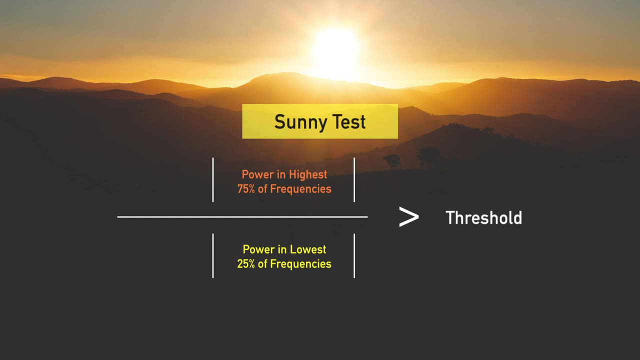 During cloudy periods, these variations can be large. Now that we've separated out the low and high frequency signals, we're ready to build our sunny test. We need to aggregate over enough time for our filters to give sensible results, but we don't want to wait too long to get an answer. 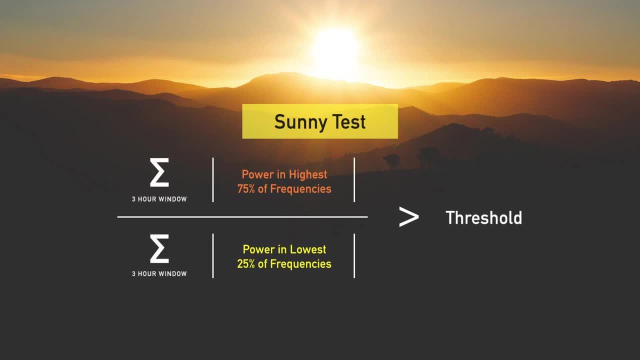 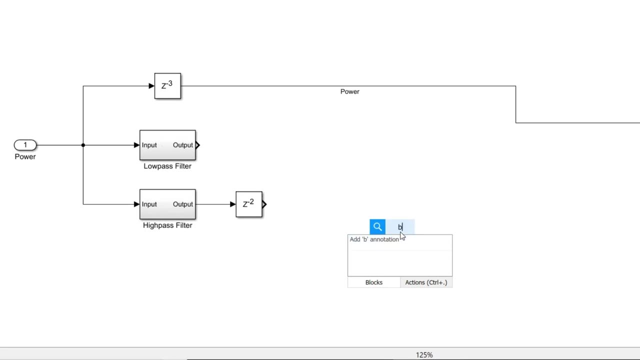 So we'll use a three-hour window, which is just 12 measurements, To store the filter outputs over a time window. we'll use a buffer block from the DSP System Toolbox. We can set the buffer size to 12 to handle a three-hour window. 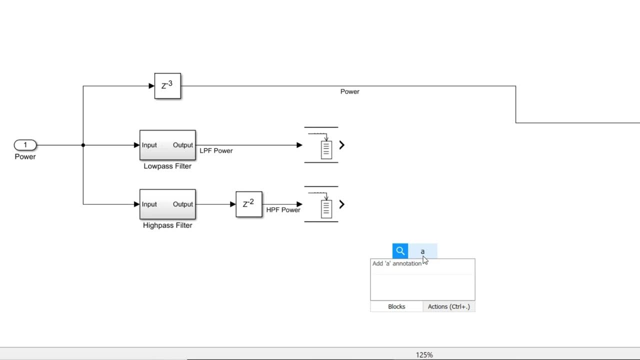 And we need a buffer on each filter path. Now we'll use some basic math: operation blocks to compute our sunny test, like the absolute value sum of elements, and divide blocks. Let's add a block to compare the ratio with a threshold. 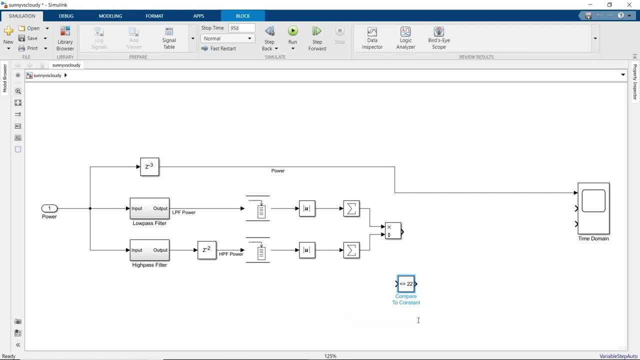 With Simulink you can experiment easily to find a good value for the threshold. 22 works well, but feel free to play with this value and see how it changes the results. The output of the comparison is 0 for not sunny and 1 for sunny. 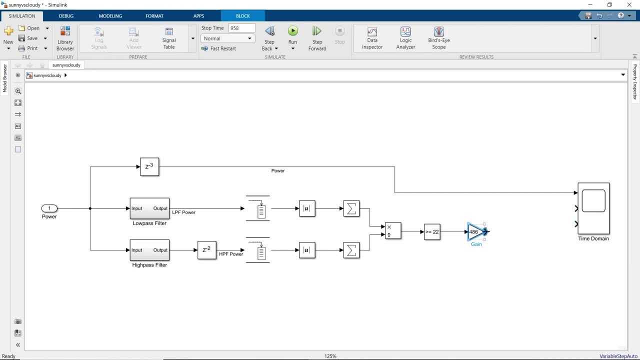 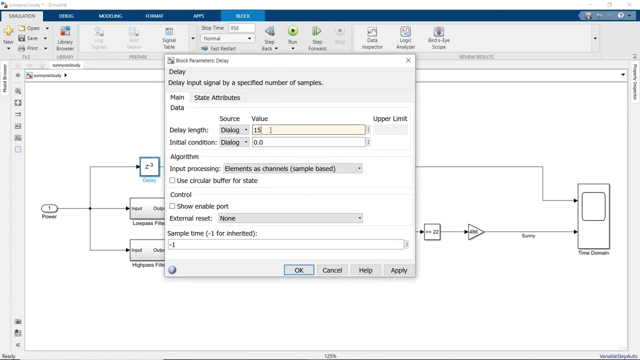 Let's scale it to match the maximum power, just so it shows up nicely on our plot, And we should remove the extra input port on the scope block Before we run. note that those buffers added some more delay to the signals. So to stay aligned with the original signal we'll need to increase that delay by 12.. 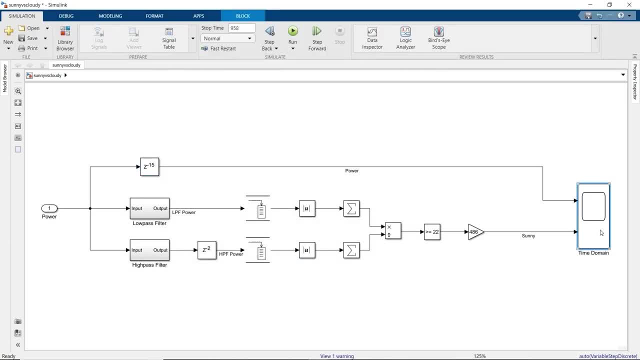 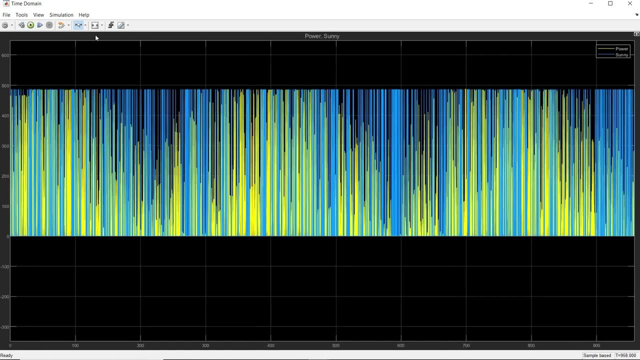 Okay, let's run and see how well our algorithm works. If we zoom in on the same days as before, it looks like it's working pretty well, But if we look at a different set of six days, we find a problem with our method. 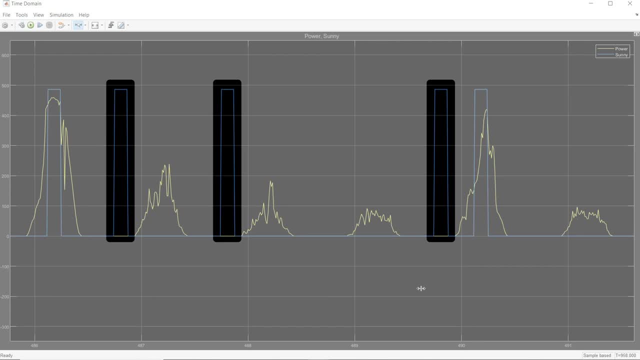 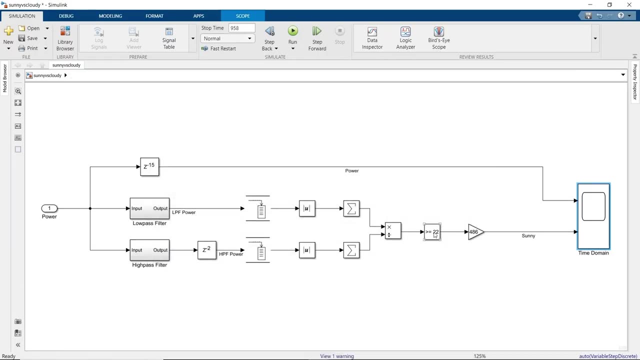 Sometimes it says it's sunny in the middle of the night. To solve this problem, let's make sure that our algorithm has a similar result. Let's modify our sunny test by adding a daylight detector. We'll simply compare the low frequency power to another threshold, which lets us know if